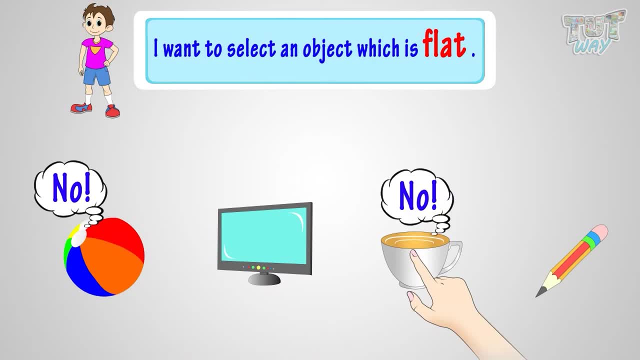 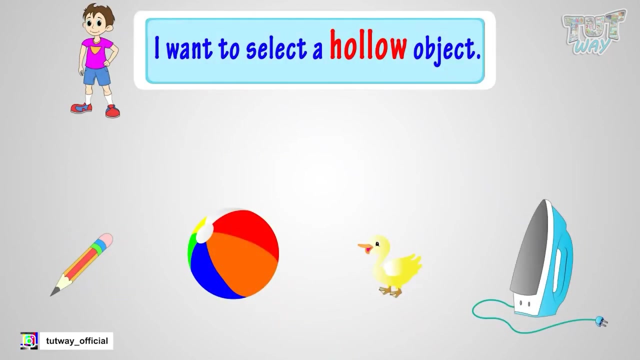 Should I choose a mug? No, It's not flat. Should I choose a pencil? No, It's not flat either. Should I choose a television? Yeah, This is a flat object. I will choose this one, Thank you. Now I want to select a hollow object. So which object should I choose? 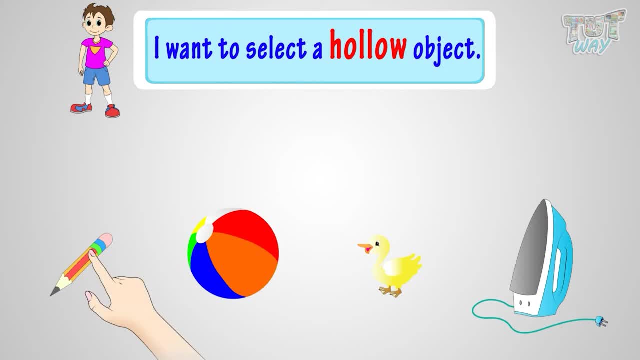 Should I choose a pencil? Is it hollow? No, It's not hollow. Should I choose an iron? No, It's not hollow. Should I choose a ball? Yeah, Ball is hollow from inside. That is, there is some empty space in the ball. 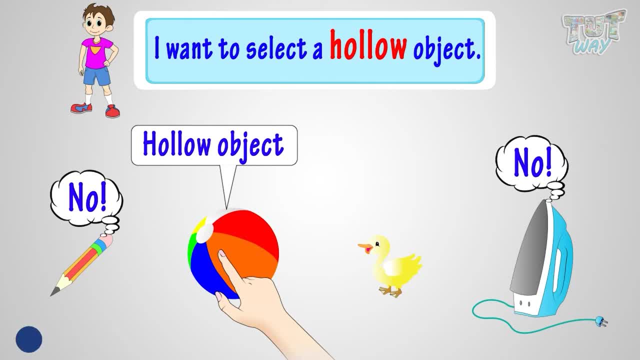 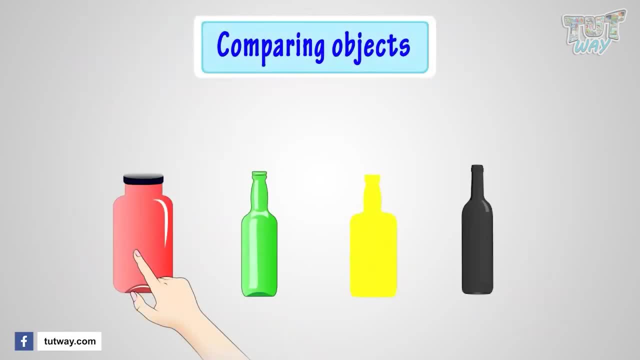 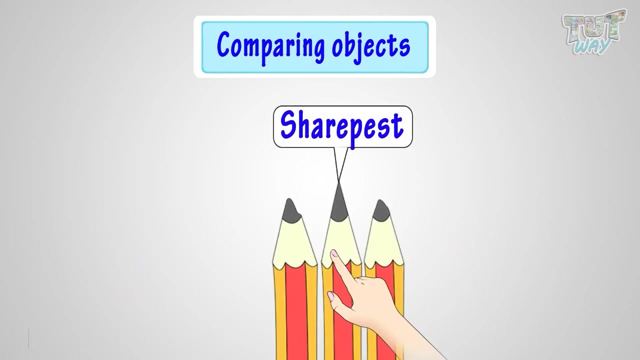 So I will select the ball, Thank you. So what have we learnt? We have learnt that red bottle has the widest neck amongst these bottles. Purple candle is the widest amongst these candles. Second, pencil is the sharpest amongst these pencils. 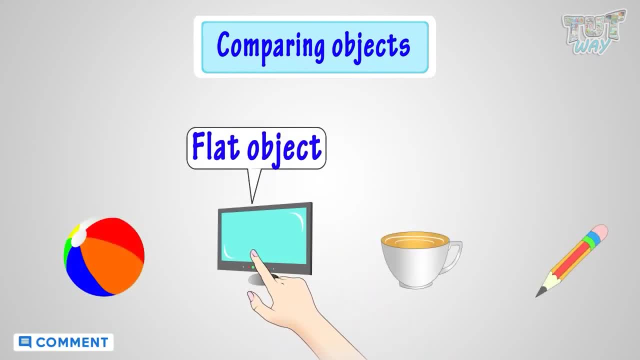 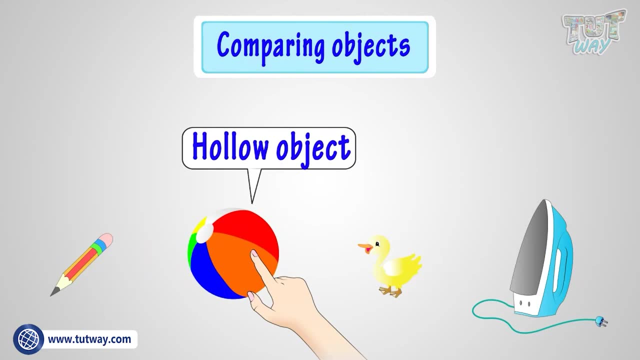 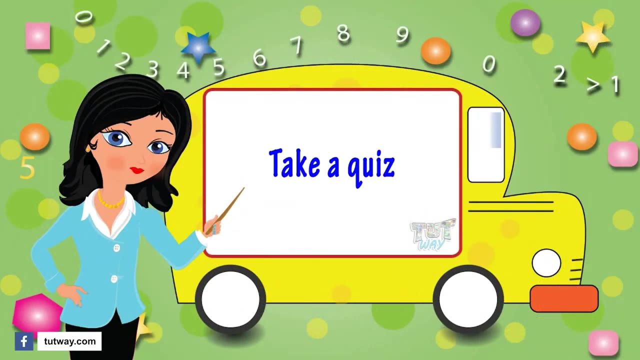 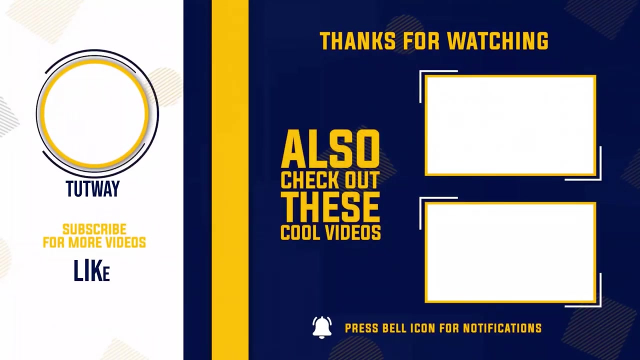 LCD screen is a flat object amongst these. Ball is hollow object amongst these. Good, Now you may go ahead and take a quiz to learn more. Bye-bye, Thank you so much for watching. Don't forget to like, comment and share this video and if you want to see more fun videos, 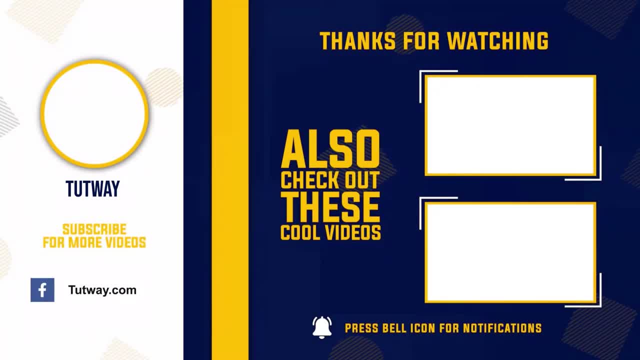 you can hit that subscribe button. You can also follow us on Facebook and Instagram for more content. Bye-bye.